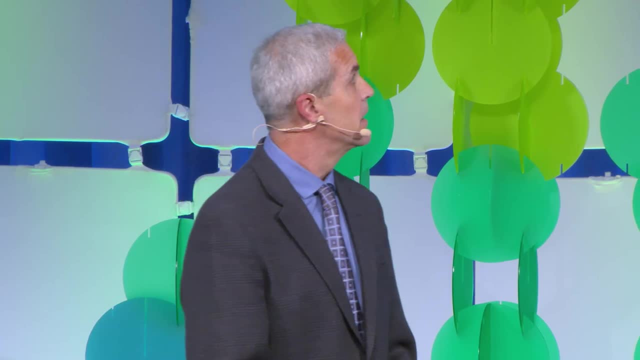 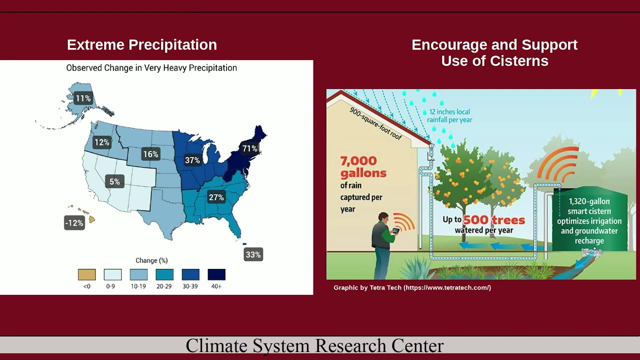 employing to handle some of these changes. So in the Northeast US we're seeing approximately a 70% increase in the heaviest precipitation events. So think, for example, the number of days each year where we see one inch of precipitation or greater, Typically in the 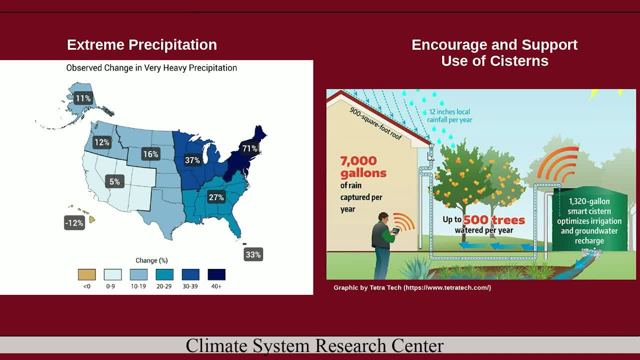 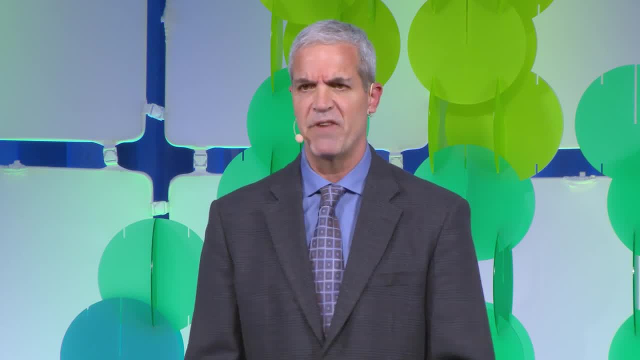 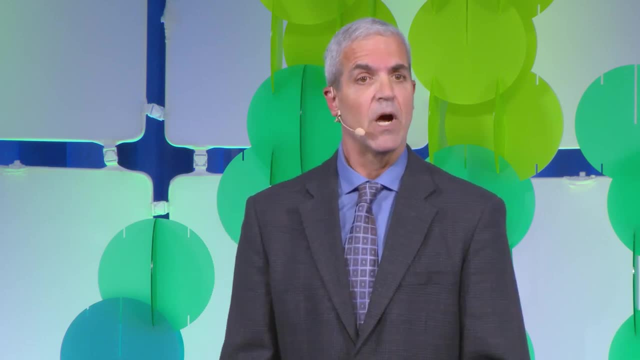 past we would see something like maybe 10 of those events each year. Well, now in the Northeast US we're seeing approximately maybe 17 of those, a 70% increase in those events, the greatest increase of any region of the US. We're wet here and the climate's warming. 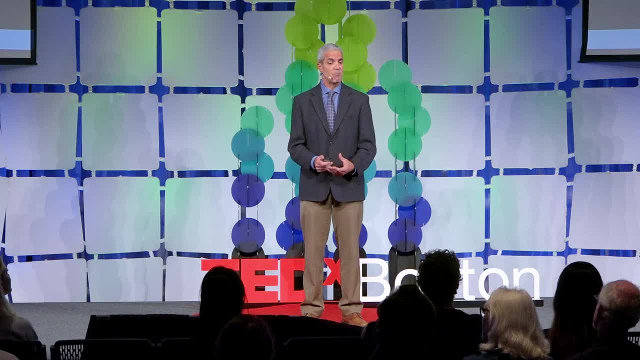 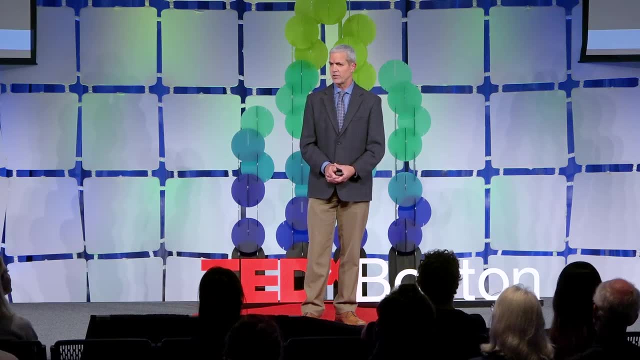 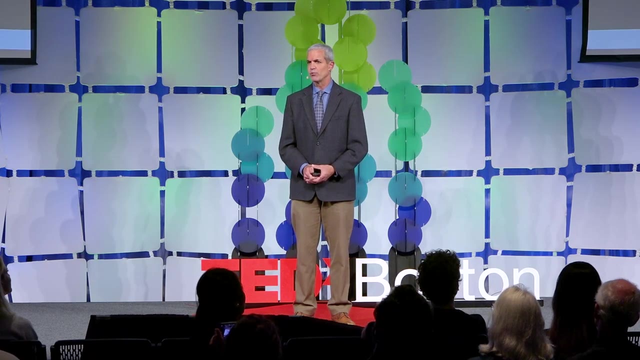 A warmer atmosphere can hold more moisture, So we're seeing a big increase in extreme precipitation events, And one of the things we can do to adapt to this is the use of cisterns. Okay, So cisterns capture runoff from impervious surfaces and direct it to a storage, So in 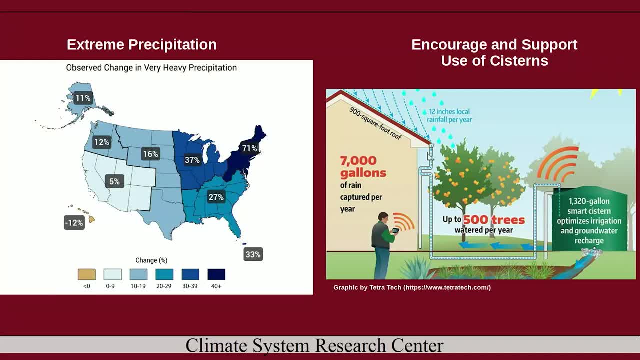 the example here we see a roof that's approximately 900, let's say 1,000 square feet can capture around 7,000 gallons of rain each year, And that's for an example where we see 12 inches of rain each year. In the Northeast US we see about four times that amount. So a typical roof that's about 900 or 1,000 square feet, can capture upwards of about 30,000 cubic gallons a year. Now that's not all the domestic use of most households, but it's a large fraction of that. So these cisterns can direct some of this runoff from roofs and impervious surfaces. 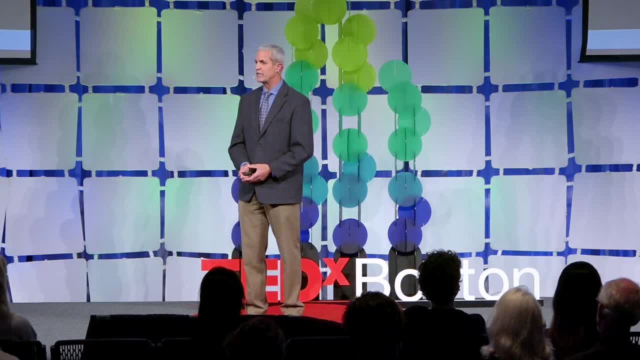 and direct it to a storage instead of it going into runoff in streams and then end up in a, let's say, or sewers and end up in a treatment facility, where it has to be. we have costs, we have energy uses to process all that water. 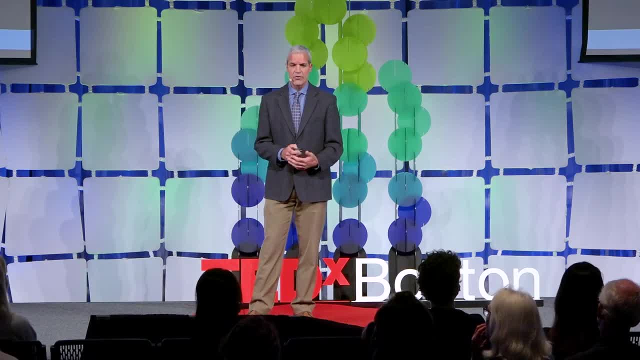 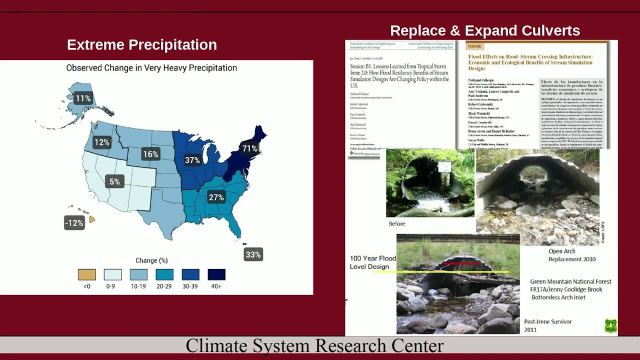 So it's really important to store some of that water. And another example of adaptation in the Northeast US is the use of culverts. Okay, culverts are where roads and rivers intersect, And in the Northeast US- well, in New Hampshire alone- there are approximately 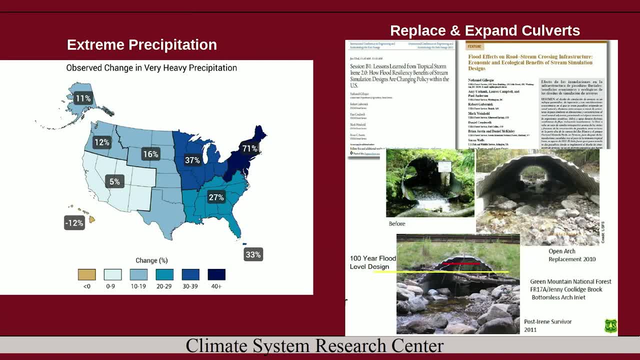 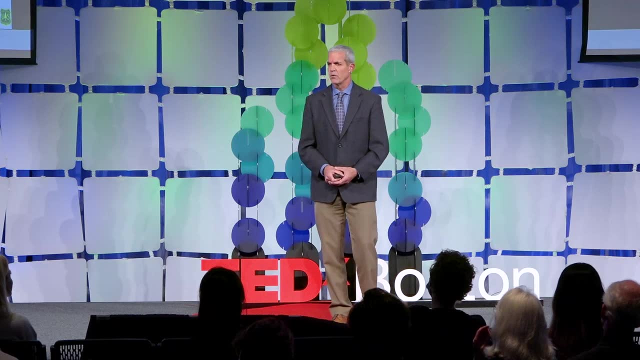 20,000 stream crossings And with an increase in precipitation and increased flooding, we need to expand these culverts. I was part of a project supported by the Massachusetts Department of Transportation a few years ago where we looked at what we can expect in the future for extreme precipitation events in 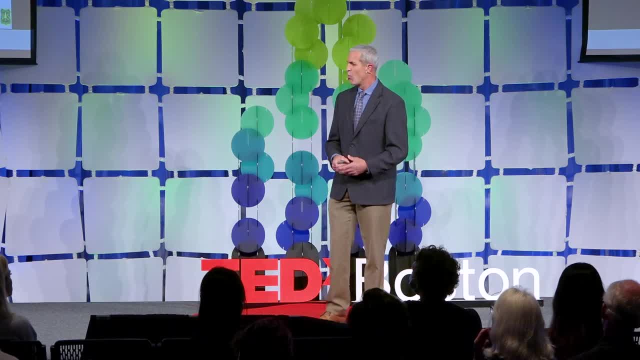 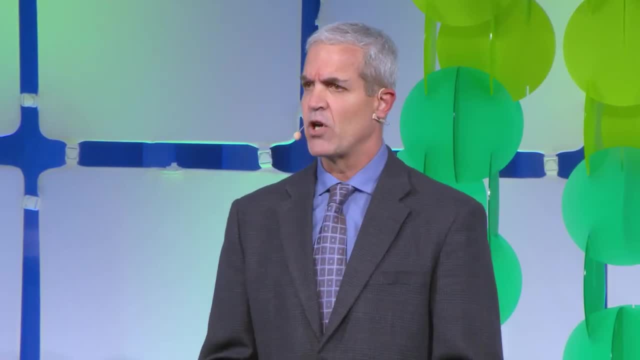 the Northeast US, how big these flows are. and then, what sizes do we need for these culverts? How big do they need to be to account for this flow, Because it's really important? these culverts have to be sized correctly, because if they're 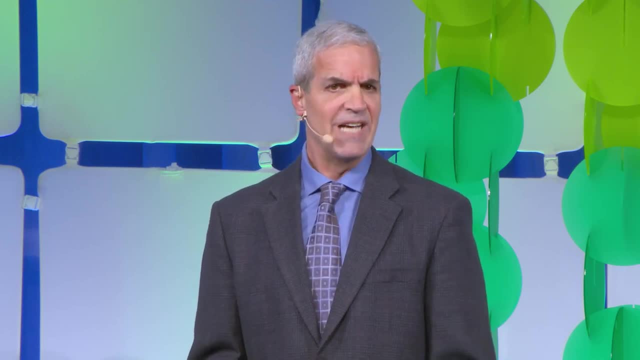 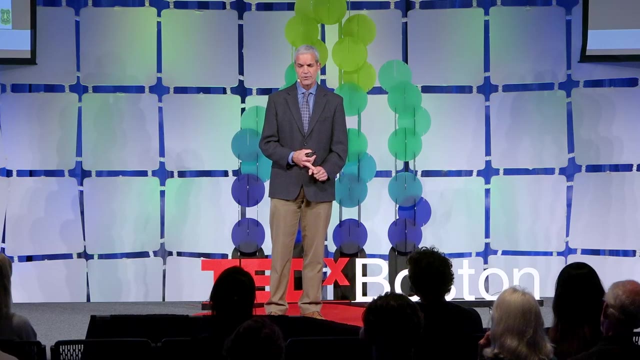 too small, that increases the flow, the velocity in the culverts and that leads to erosion and sediment transport, And that's really problematic for aquatic animals. So a culvert needs to be as wide as the riverbed. Ideally it's arch-shaped And also ideally. 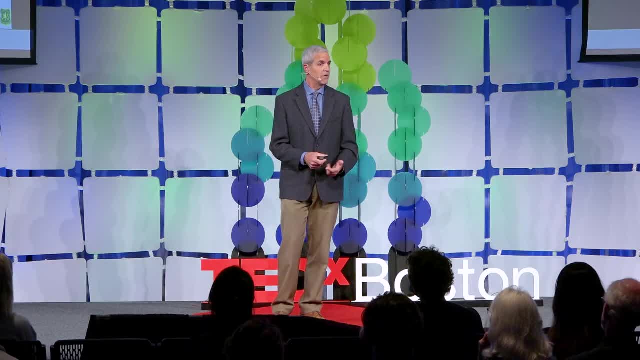 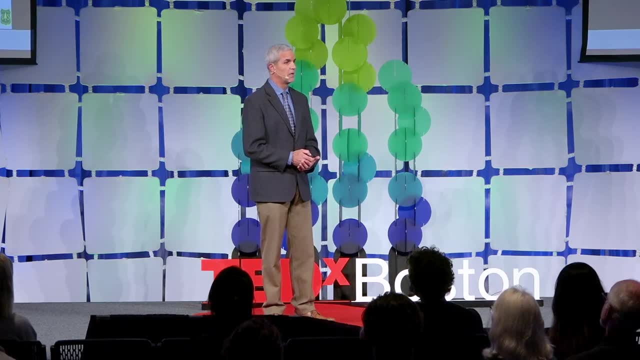 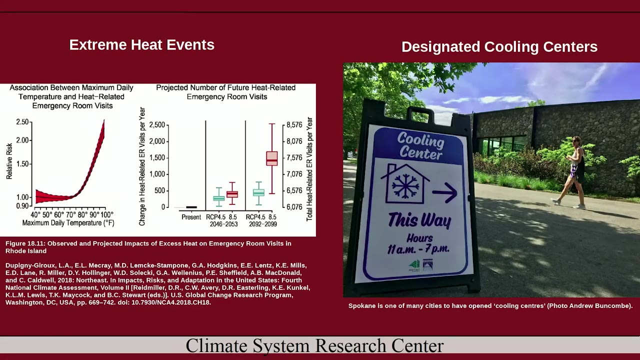 it has a natural bottom to allow for movement of aquatic organisms, So it's really important to think about culverts and expanding those. as the climate warms and we get increased hydrological flows, extreme precipitation events- We're also seeing extreme heat events in the Northeast US and other parts of the world, obviously, So the 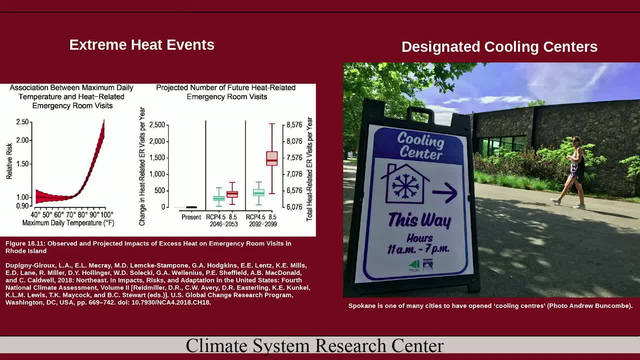 association between extreme heat events and emergency room visits is notable. It's significant. So once we get up near about 90 or 100 degrees Fahrenheit, we see about a doubling of the risk of emergency room visits, And in the future. this was an example from a study for the state of Rhode Island And, in this example, under the highest emission scenario. in the future we might see a number of increased visits and emergency rooms under the highest emissions scenario by the end of the century, anywhere from about 6000 visits a year to upwards. 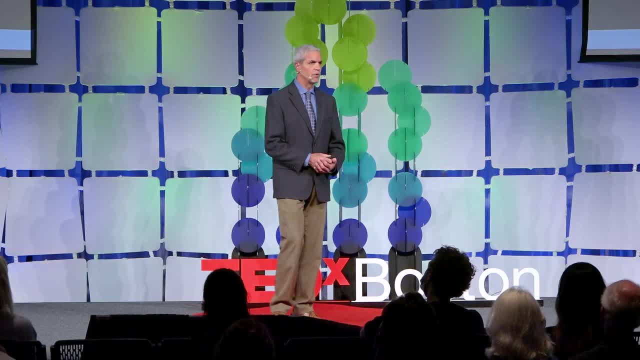 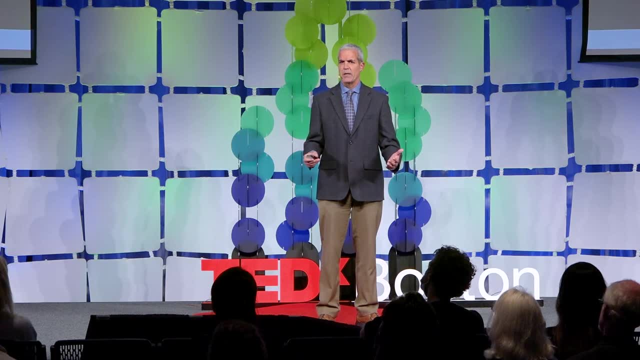 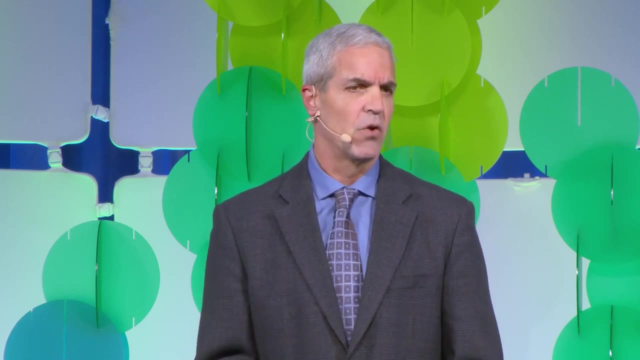 of 7500.. Cooling centers are a really, really important part of adapting to climate change. Cooling centers: we need to obviously understand where our vulnerable populations are. take a look at where the resources should be deployed. Are these cooling centers located in the right areas? Do they have enough resource locations? 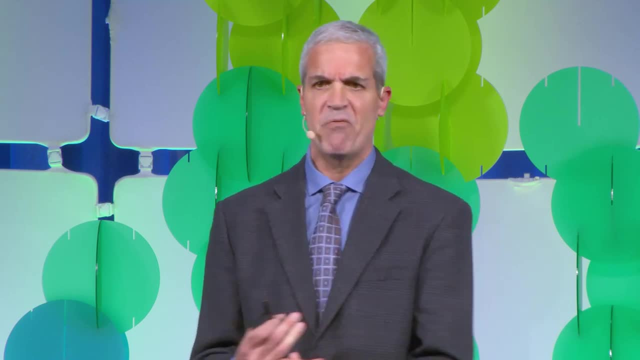 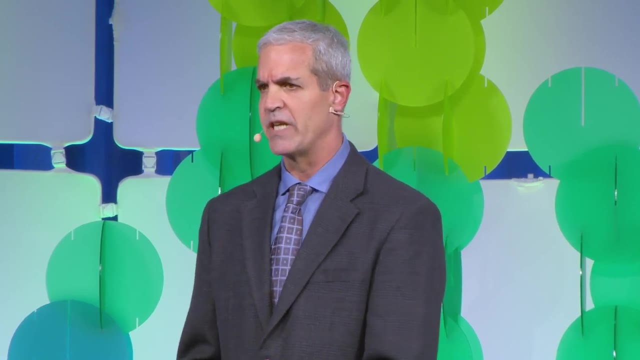 Are they worth corn? Anyways, all those factors sup 채 resources. Is there enough public information about where they're located, when they're open? Can we use things like malls and schools, air-conditioned areas to protect our most? 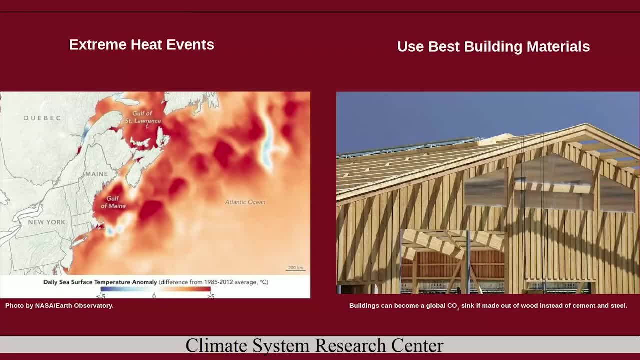 vulnerable populations Really important. Some of these extreme heat events in the northeast US are driven by not only warming being forced by increasing greenhouse gas concentrations right directly on land, but also the warming in the western Atlantic we're seeing. So this was an anomaly from a couple of years ago that showed extreme warming in the western 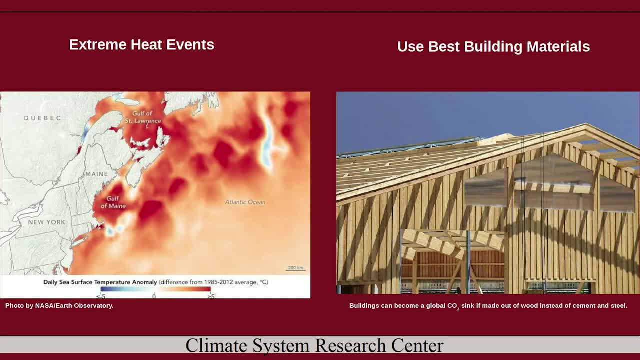 Atlantic an anomaly, so a departure from an average condition here in a departure from the 1985 to 2012 average showing the warming in the western Atlantic And, interestingly, a study that was published in Nature just a few years ago showed that the warming in 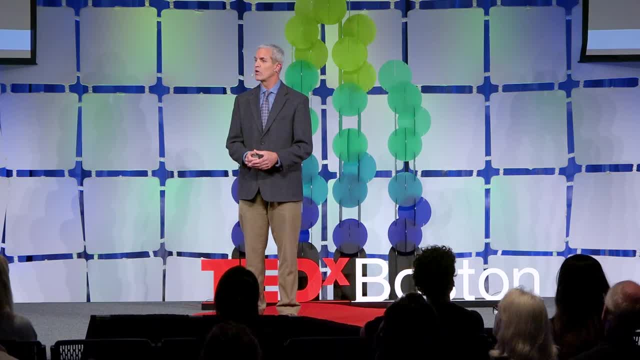 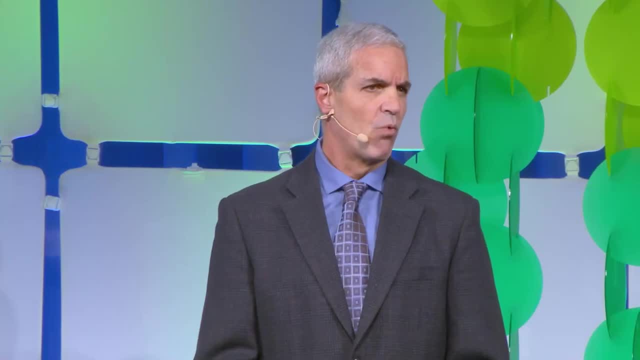 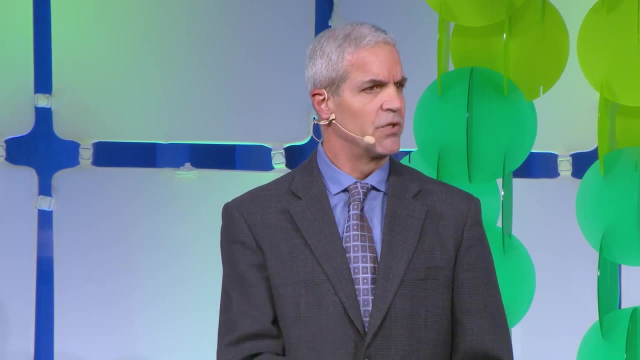 the northeast US is highest, closest to the coast, And the author of this study, a colleague of mine at US Amherst, determined that some of this warming along the coastal regions is due to atmospheric changes in the atmosphere, but also due to this warming in the western Atlantic. So the 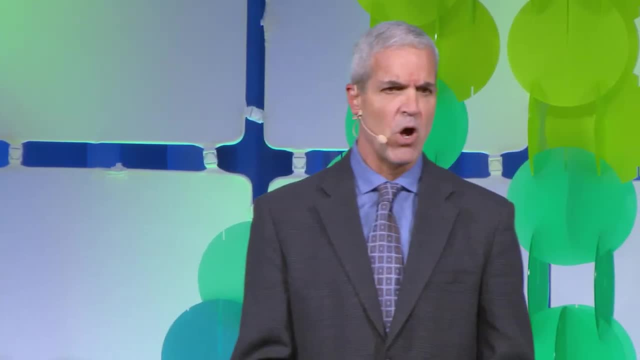 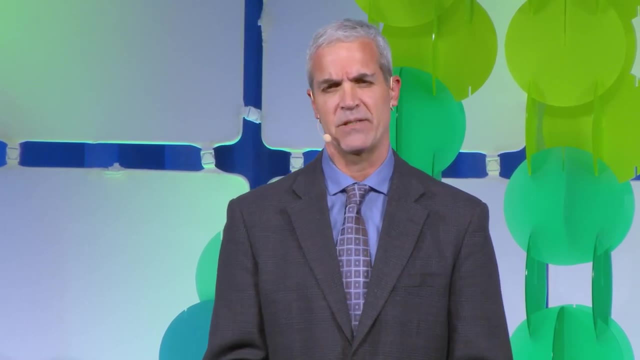 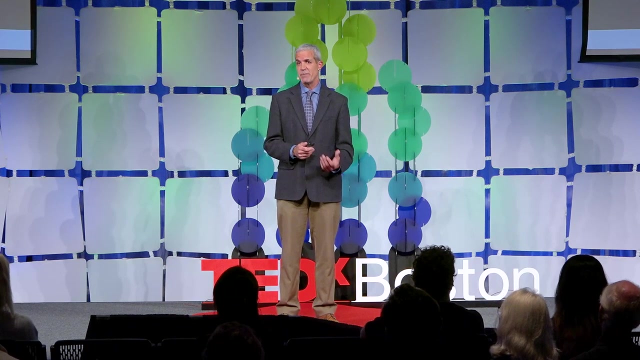 western Atlantic is getting warmer and warm. ocean water holds a lot of moisture, holds a lot of water and heat and doesn't dissipate as easily as land does. So building materials are really, really important to understand. okay, can we limit the extreme heat stresses? 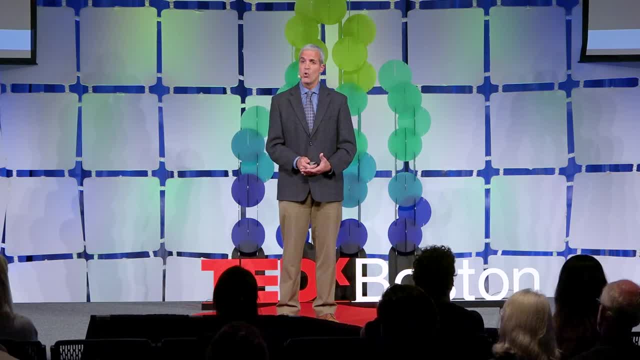 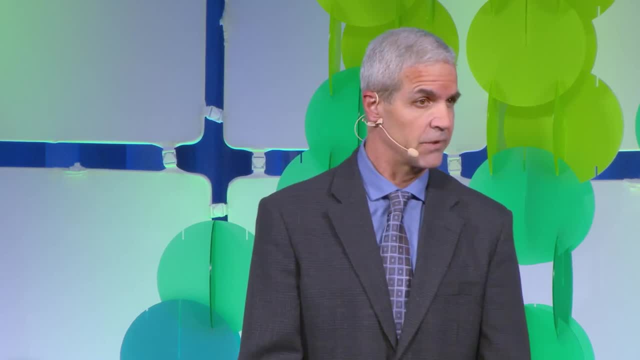 we're seeing. Can we limit the extreme heat stresses we're seeing in our populations by using wood instead of brick and concrete? As you know, making of concrete is one of the major contributors of greenhouse gas emissions. So if we go to using things like wood, wood can actually 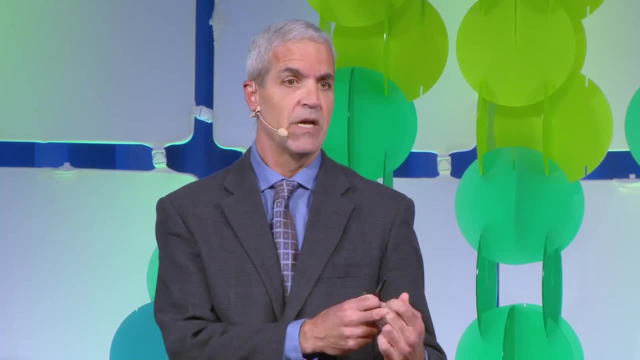 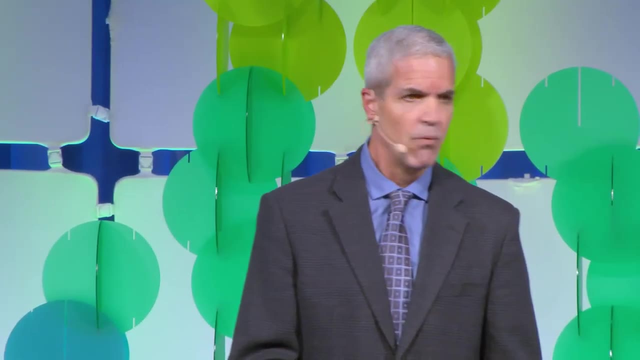 sequester carbon. It's inert and it's as long as we sustainably grow our forests. So important use of building materials. We don't want to use brick anymore because brick holds the heat in. There were approximately 20,000 tons of brick in the US in the 1960s and 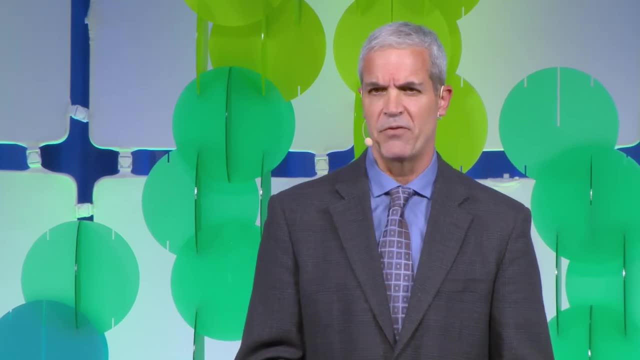 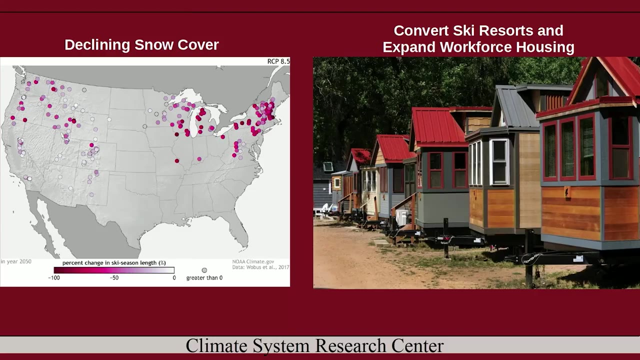 there were approximately 20,000 or 30,000 deaths in western Europe a few years back, about a decade ago, in an extreme heat event. Brick apartments are really really problematic. Declining snow cover is another issue in the northeast US, So it's getting warmer Winters. 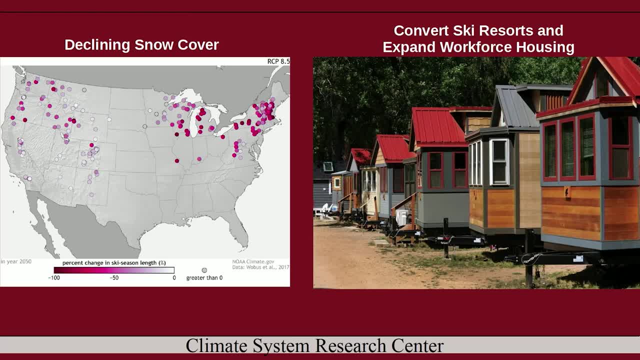 are getting warmer, We're seeing declining snow cover and, particularly in the northeast US, probably larger declines than any other part of the US, Upwards of 60,, 80, almost a 100 percent decline in the ski season. 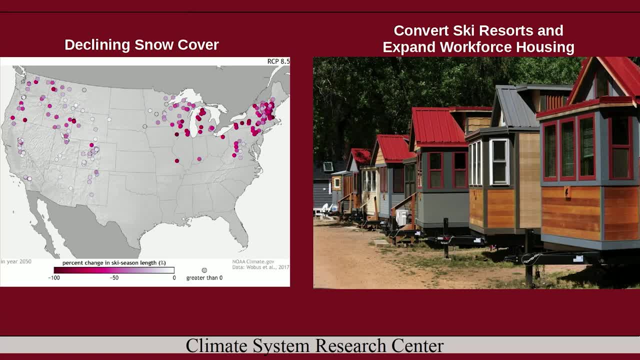 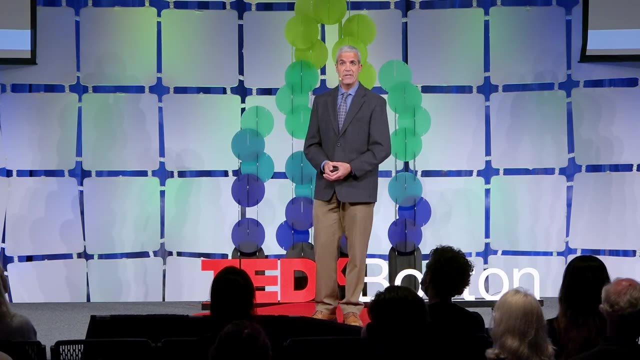 So do we need to repurpose and think about some of these ski resorts and maybe using them for—or hoping that they get converted to warm weather recreation And the housing that's there, the lodging, the apartments, the condominiums? maybe they should be repurposed. 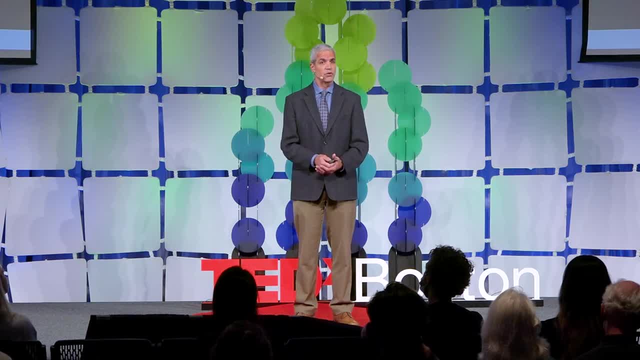 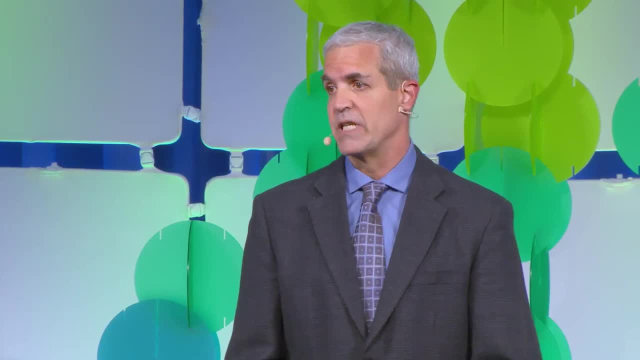 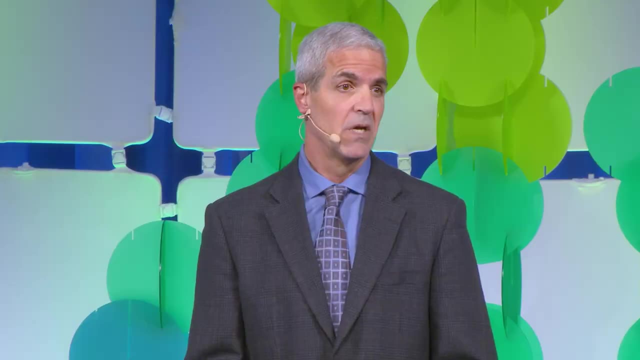 and used for housing of workers. And then how about small houses, tiny houses, Using them for workers in that area? ski resorts in the Northeast US, in the southern parts of the Northeast, probably are going to have a big problem sustaining themselves as snow cover. 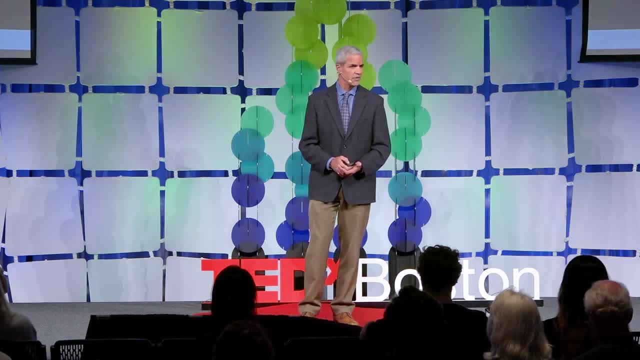 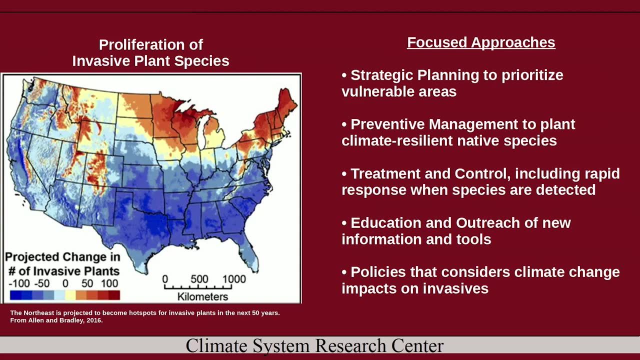 declines, we can still make snow, but it's hard to make snow when the temperatures are above freezing. invasive species are proliferating across the Northeast US, more so than perhaps any other part of the US. approximately a 100% increase is likely toward the end of the century in the case of a high submission scenario. 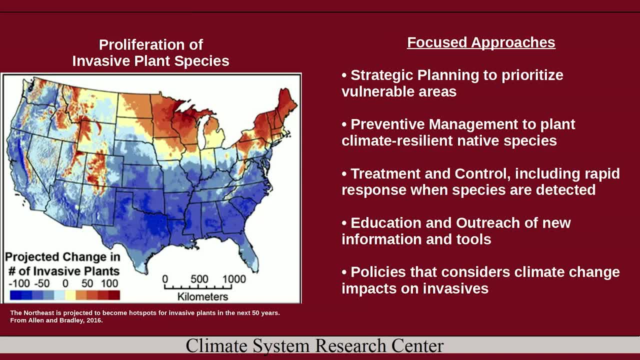 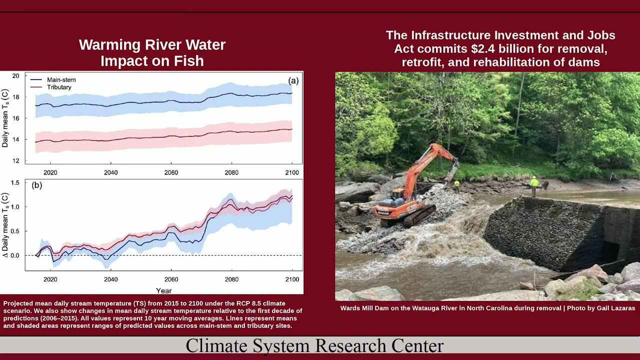 so what can we do? as far as invasive species, we got to think about strategic planning, preventative maintenance management. when these invasive species show up, we need to have treatment and control. education and outreach is really, really important, and then policies that consider climate change impacts on these invasive species need to be taken into account. how about warming of river? 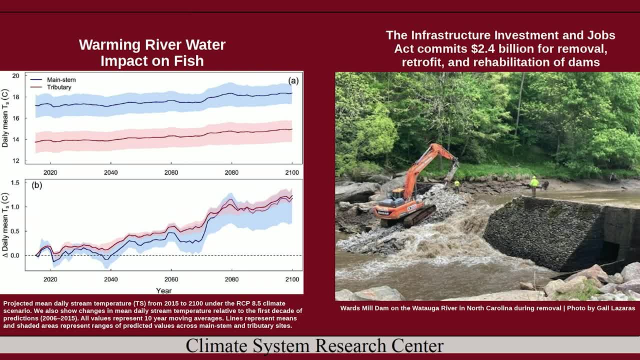 waters and their impacts on fish. so brook trout in particular in the Northwest US is one of the most important species in the United States and we've had a lot of problems with the river water in the Northeast US are seeing a lot of increased stress due to the warming rivers in the Northeast. 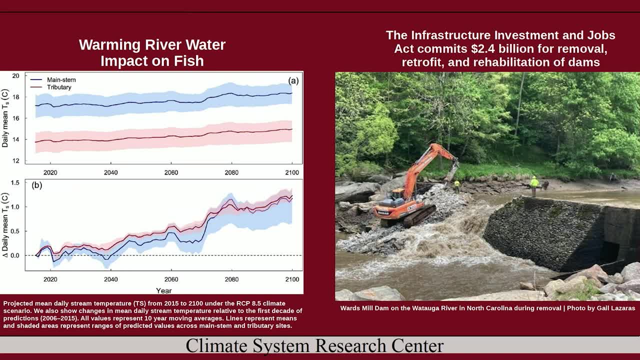 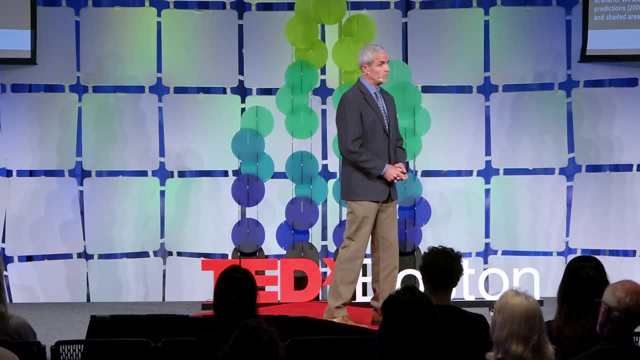 here's an example from a study published recently that shows by the end of the century, under the higher emission scenario, perhaps a 1 degree Celsius increase in river water temperature. well, there's not a whole whole lot we can do about the river warming, besides mitigating our use of fossil fuels. but 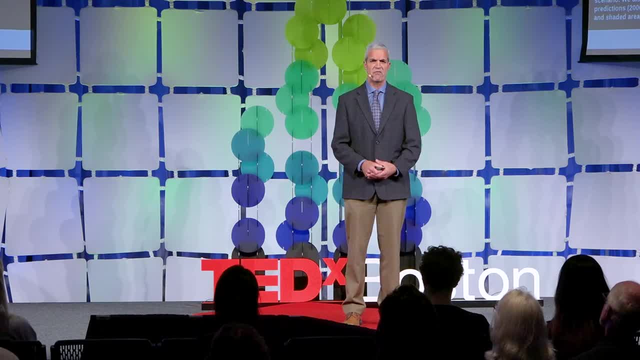 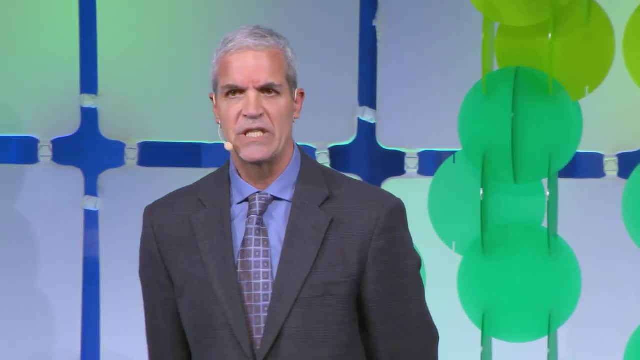 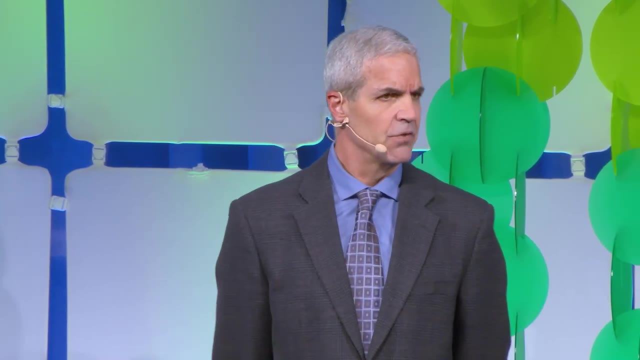 we're also looking at the natural flows in the rivers. there were approximately a little over 50 dam removals in the US last year and it's likely in the next few years we'll see that increasing. there was approximately, with those dam removals, a restoration of around 2,000 miles of rivers to their natural flows. 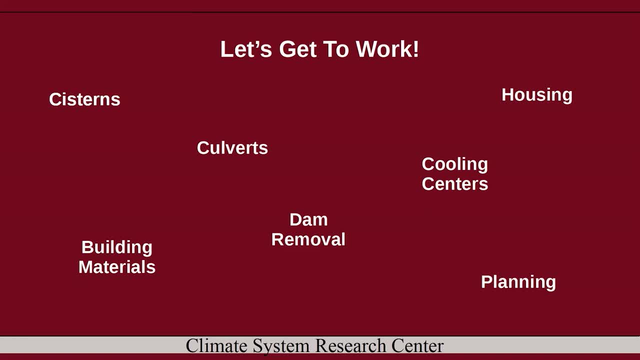 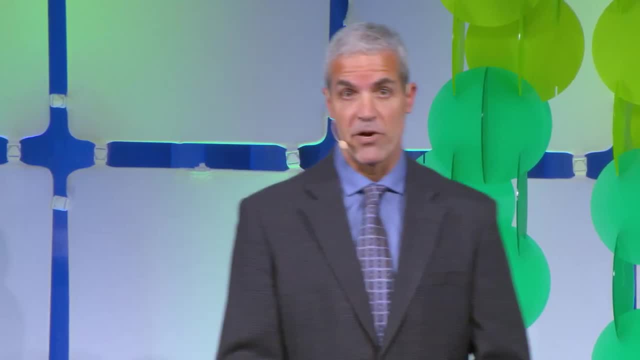 the investment infrastructure act that was passed allocates around 2.4 billion for the removal, retrofit and rehabilitation of dams. so let's get to work, thank you.